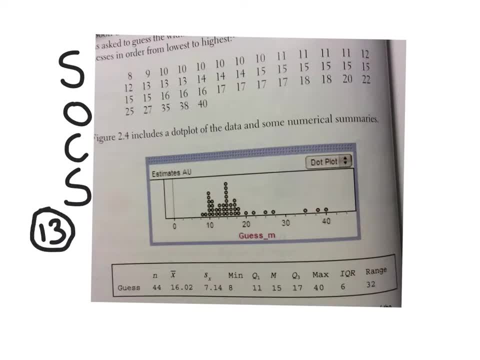 So if we subtract 13 from every one out of these data points, it tells you what their error was. How far were they off? So, like this kid was off by 3, okay, This guy was off by a negative number, okay. 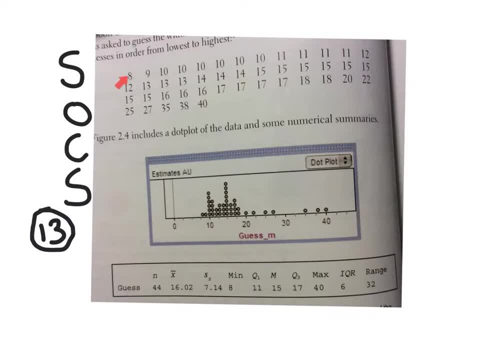 In the other direction. Still off by what? 5, negative 5.. So that's what they do. Subtract 13 from all of these. Now, what does that end up doing To our dot plot? Does it look the same or is it going to look different? 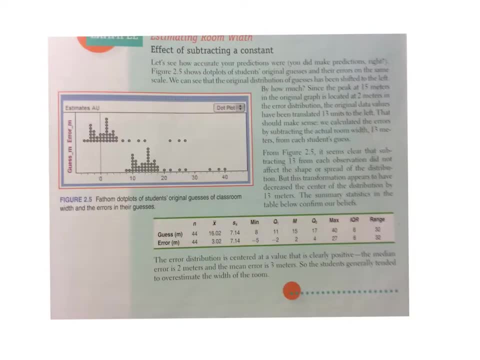 And in what way. So what we do is we take 13 away from all of the numbers, And they're nice because they show you right here. Here's the original numbers, right? And this is after you subtract 13 from everything, right? 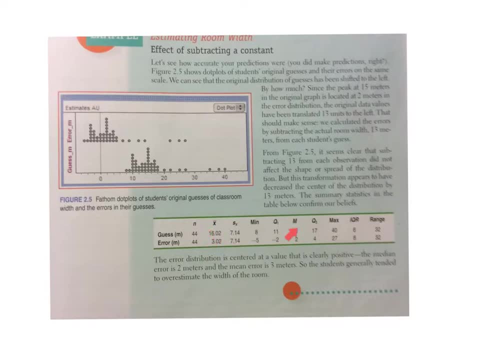 Take 13 away from the average, Take 13 away from each one of those numbers. So it's basically going to take the exact same, the exact same graph- here's our original- and just kind of slide it down, okay, by 13.. 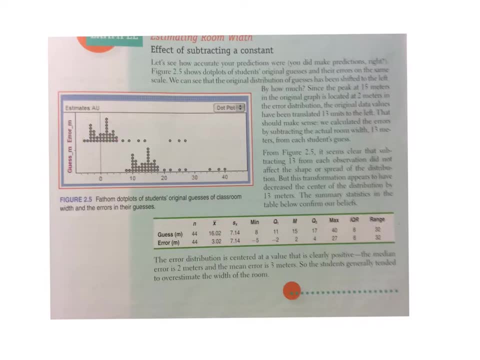 The shape doesn't really change. okay, It's still spread in the same amount. So, in other words, the inner quartile range won't change. right, The range isn't going to change. The difference between these two numbers is the same. 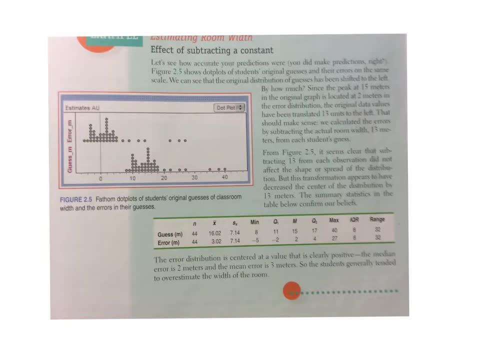 even though they're smaller. And then also the- where is it? the standard deviation doesn't change either. It doesn't stretch this thing, It just slides it down. Same exact shape, just smaller. Okay, So let's take a look at what that looks like. 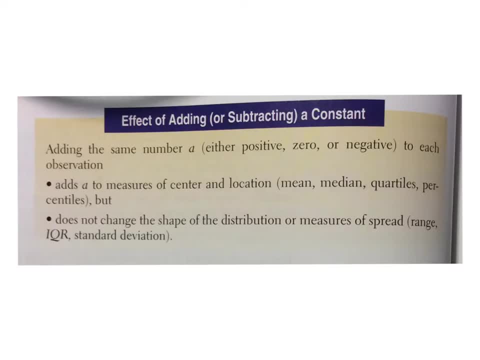 Well, I guess it's that tan box helps us, So this might be good to write down in your notes. Maybe I would let you use it on a test or a quiz Plus. it just helps you remember it when you write it down. 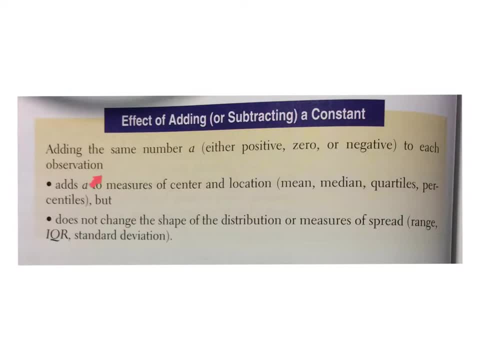 Basically, what we're saying is: if we add or subtract a number, that's A right. Well, what gets changed? The median, the mean, the quartiles, the percentiles, all that stuff gets changed, okay. So if we add, say, 20 to all the numbers, 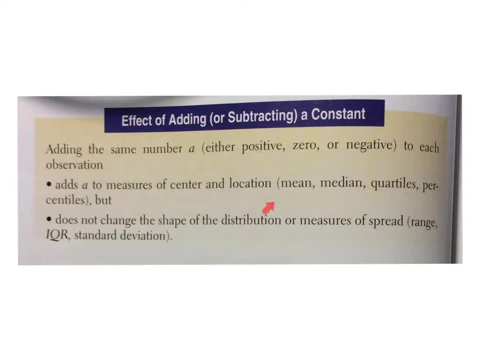 all of those get 20 added to them. If we subtract 13,, all of those go down by 13.. But what does not change? Well, what doesn't change is the shape of the graph, which means the range, the number, the number of. you know. 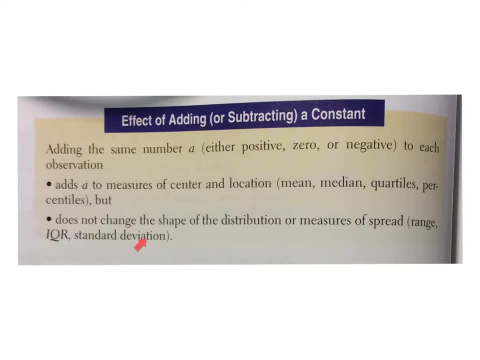 the range, the inner quartile range and the standard deviation will not be affected, because we're not stretching it or shrinking it, We're just sliding it in one direction or the other. Okay, Hopefully that helps. Let's talk about when we multiply. 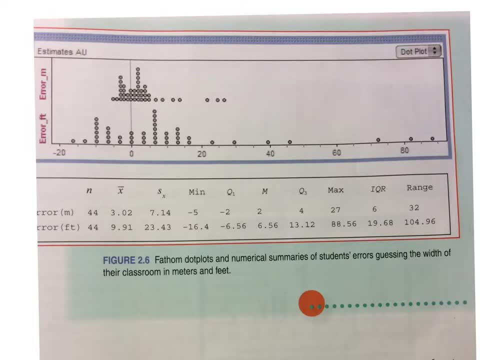 So in this one they took that second graph, the one where they subtracted 13 from all of them. So this is their error in meters. And they said, well, what if we just translate it into feet? Well, it turns out there's about 3.28 feet is equal to one meter. 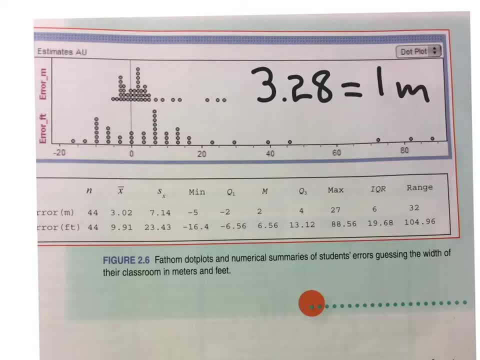 So what they had to do is take each of these numbers and multiply it by 3.28.. So the minimum negative 5, multiply it by 3.28.. That's where that negative 16.4 comes in. okay, 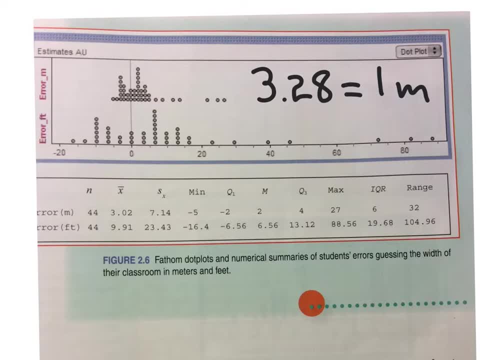 So all of those numbers get multiplied And you'll notice the result: It gets spread out. Aha, So what does that mean? Okay, So everything gets multiplied by that 3.28.. It stretches it. The bigger numbers get bigger. 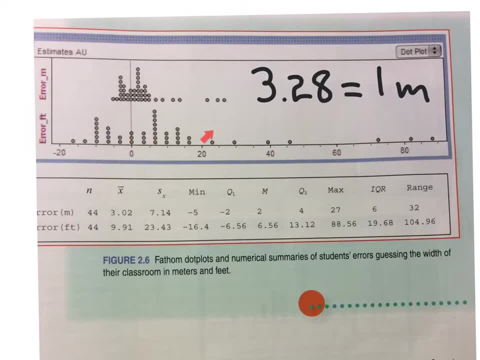 The smaller numbers get smaller And it stretches it out. If we were to divide by a number, it would make it narrower, Okay, But let's just talk about stretching this thing out. What does that mean? Well, that means that everything gets multiplied by 3.28.. 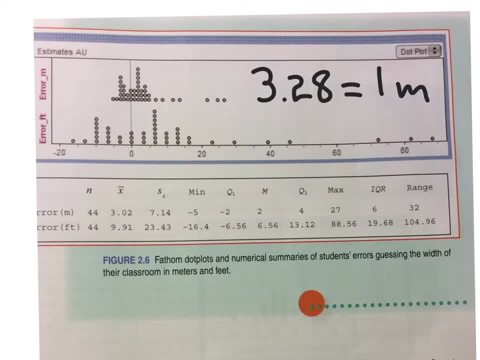 Even the standard deviation, the interquartile range, everything gets multiplied by 3.28. when you multiply by a constant, The only thing that doesn't change is the shape of the graph. It's still skewed to the right, Still has these two peaks like this: 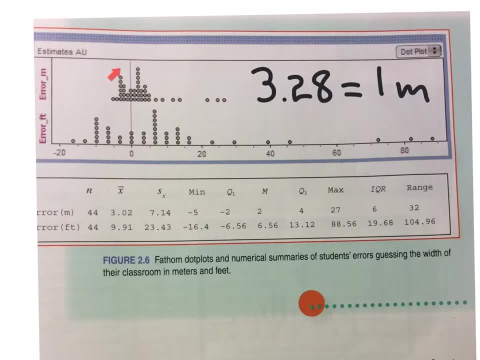 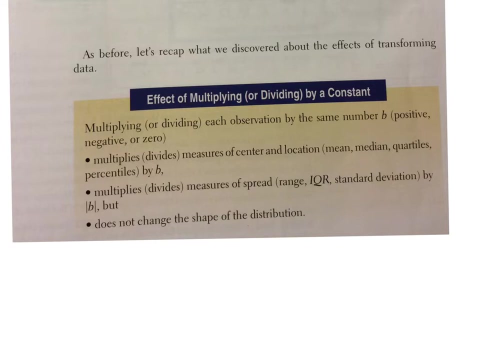 It's still the same general shape. right, The shape is the same, It's just spread out, okay. So now let's take a look at what that box says. Let's see, Right, And here again, Multiplying or dividing by some number. b right.